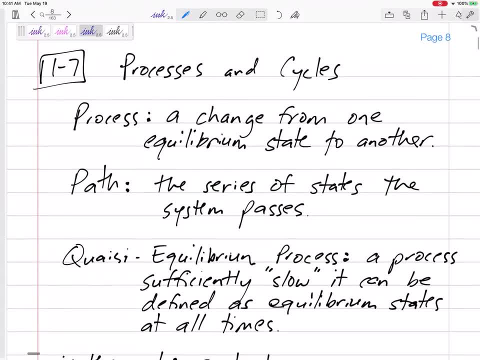 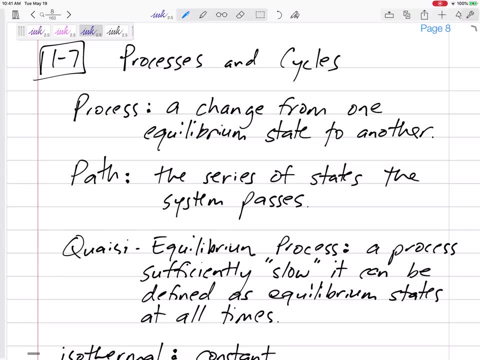 Alright, section 1-7.. Some definitions of process season cycles. A process is just a change from one state- and we're going to assume it's an equilibrium state- to another equilibrium state, And the path is the series of states that that system passes to get from one state to another state. 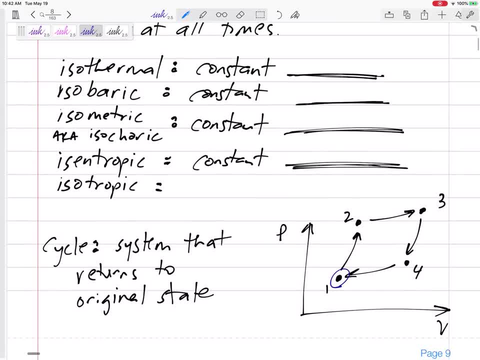 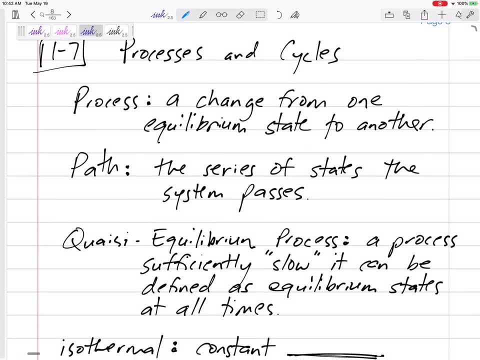 For example, we go down here One state to two state and then this path it takes would be all the different states that it goes from, from one to two. Alright, so process is a change from one state to another. A path is a series is the direct. you know the series of states that it passes. 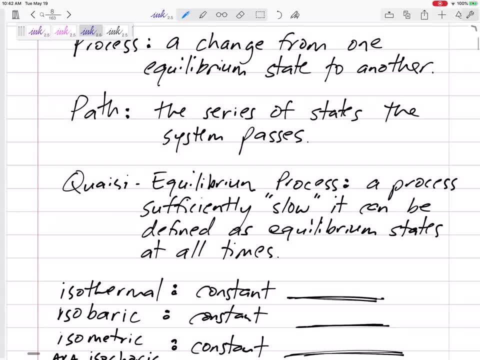 A quasi-equilibrium process is a process that is sufficiently slow that it can be defined as equilibrium states at all times. Equilibrium states, Remember it, says that the temperature is the same throughout, the pressure is the same throughout. That may not be true in a lot of high pressure, high temperature and some very fast processes. 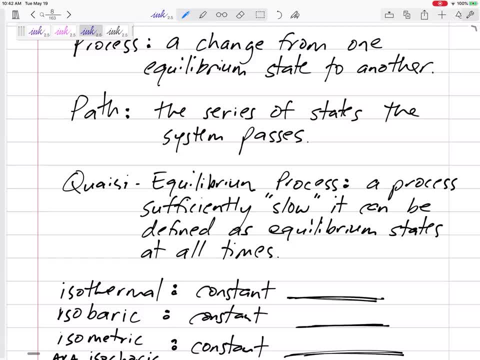 May not be going from equilibrium state to equilibrium state to equilibrium state, But in this class we're going to be looking at equilibrium process, or at least quasi-equilibrium process, to say basically every path, every state that it goes through, we're going to assume, is an equilibrium state where the temperature and pressure is the same throughout. 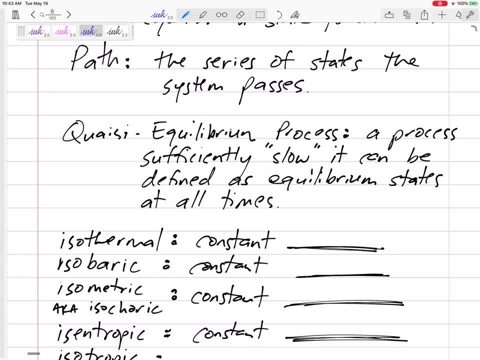 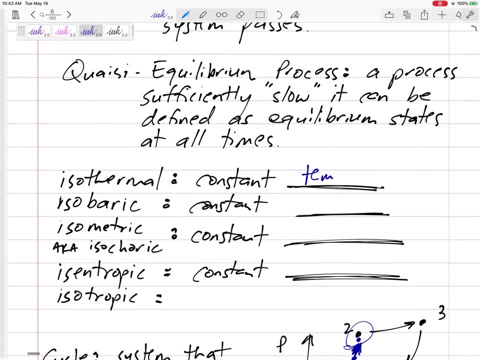 It's not like the temperature at the bottom is changing differently from the temperature at the top. We're going to assume that the temperature of the whole tank, let's say, rises at the same temperature throughout. Alright, some definitions. A process that is isothermal has a constant temperature. 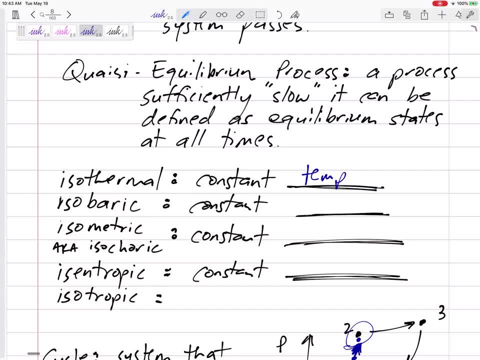 So if we're looking at a problem and it says something about you know this is an isothermal process and they give us the initial temperature, then what does that mean? That means we know the final temperature. We need to know these definitions to get all the information out as we can. 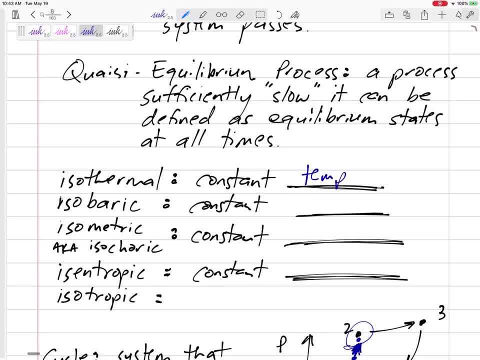 Something that is isothermal has a constant temperature. I bet you all know a lot of these, most of these. Something that is isobaric has a constant pressure. Something that is isobaric has a constant pressure from start to finish right.